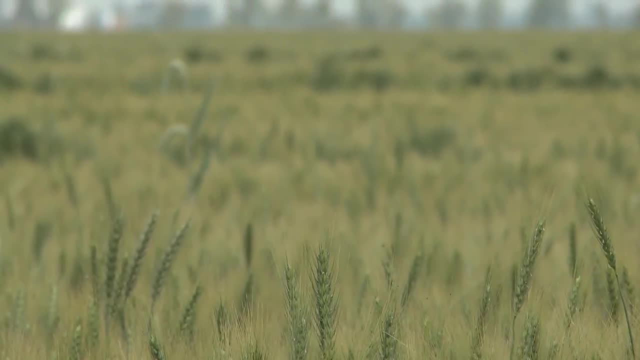 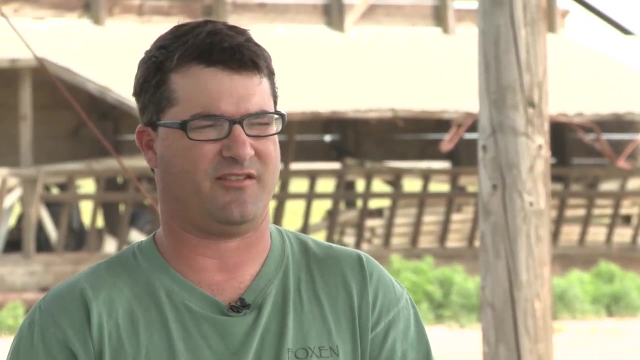 We're milking 900 Holstein cows and farming just under 1,000 acres of silage crops for the cows and alfalfa. Probably the most important things that we've learned about converting silage is that we're starting from a conventional farming system to, you know, a conservation farming system. 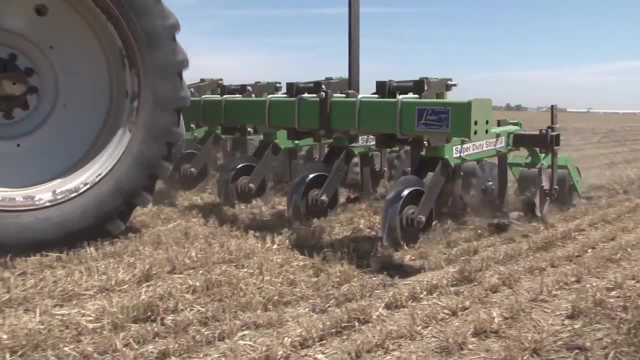 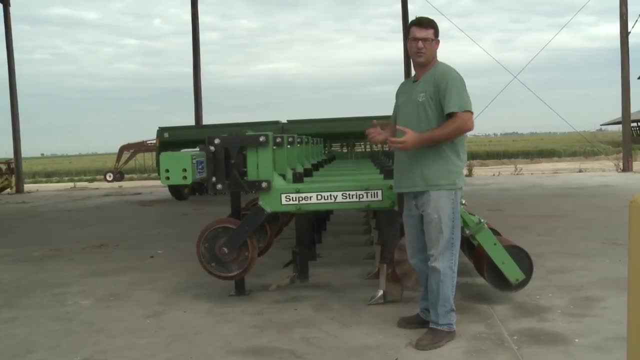 which includes strip-till, is understanding that it's a whole new system and a whole different way of thinking about farming. A strip-tiller is an implement that manages to do multiple things in one pass. It's doing sort of vertical till where you have a shank like a ripper shank that's tilling and breaking. 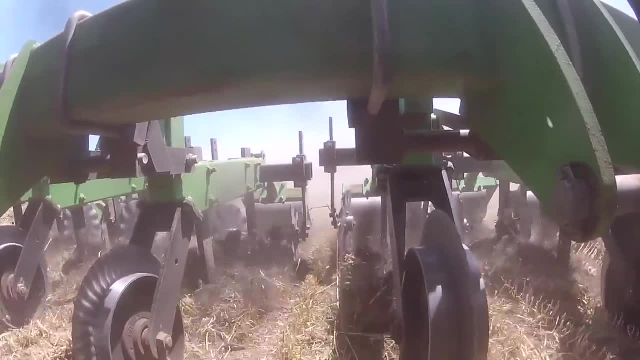 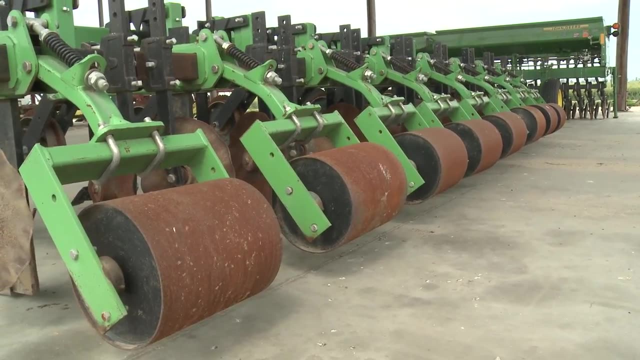 up the compaction layer. You've got these wavy coulters in the back that are shattering the dirt and creating kind of a disking type of effect, And then you've got these rollers in the back that are flattening out the strip. 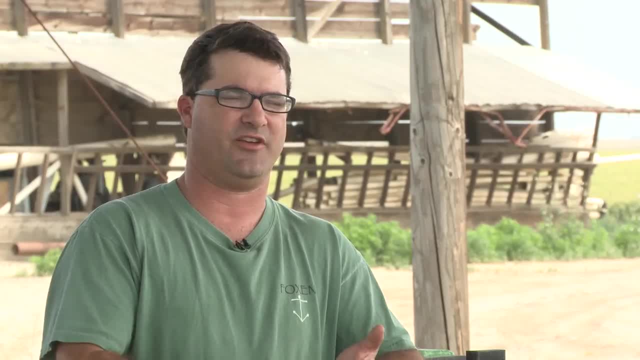 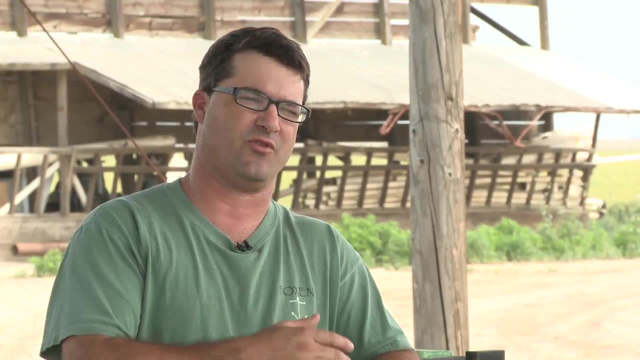 Our cycle is basically winter. wheat comes off, we strip-till, irrigate, plant corn, then we take the corn crop off, spread manure, incorporate the manure with a light disking pass and then plant wheat and that's it. 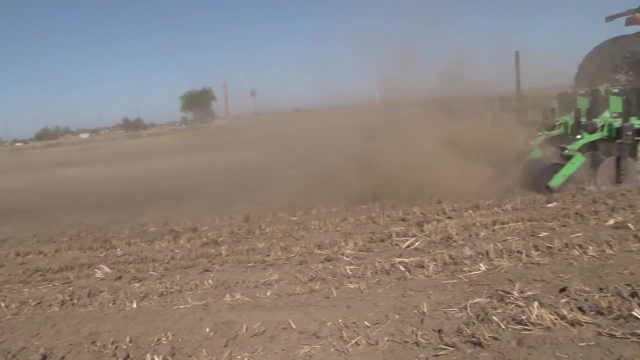 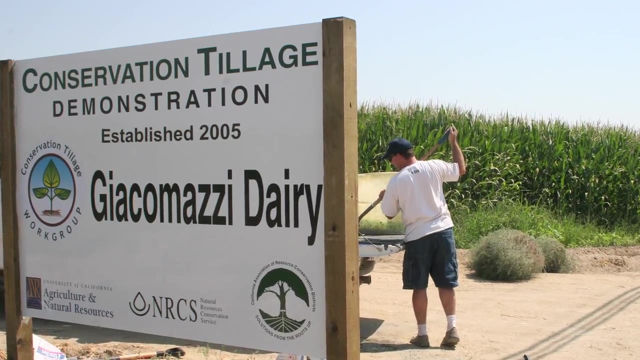 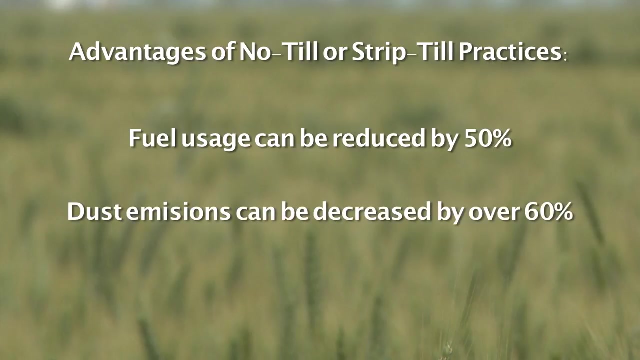 What we used to do in 11 passes we're now doing in two. That's a huge reduction. Research conducted by University of California investigators with Dairy Silage Producer Partners suggests that fuel can be reduced by 50% and dust emissions can be decreased by over 60% using no-till or strip-till practices for silage production. 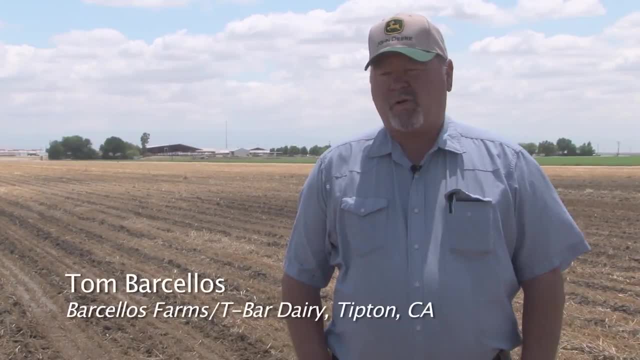 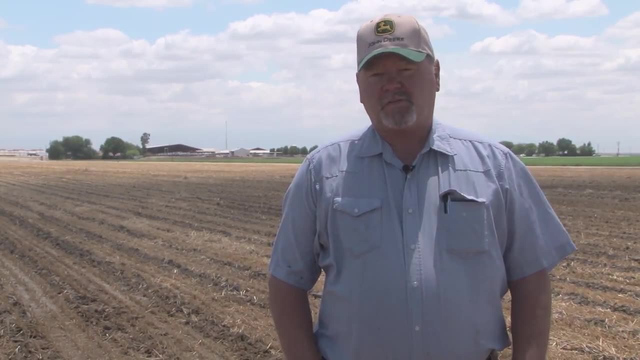 My name's Tom Barcelos. The conversion to CT programs, the way we've incorporated it, is actually very minimal. If you're going to strip-till, you can still strip-till and use a conventional planter, with maybe one minor adjustment: You may want to put a coulter. 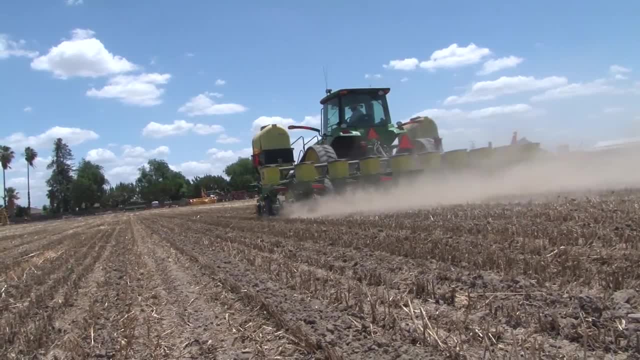 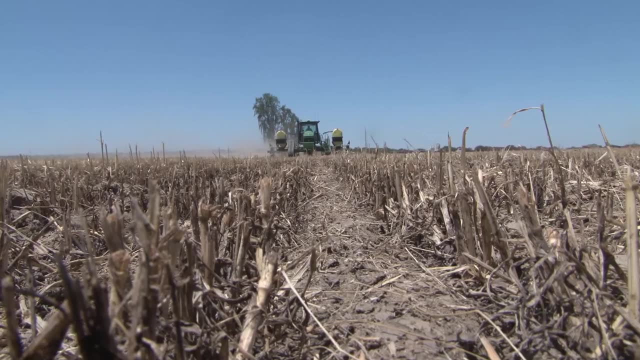 on the front of it. But we use basically the same style of equipment. We run the strip-till bar, We have our planter set up that it can go no-till or conventional, And then we also have a no-till drill. but 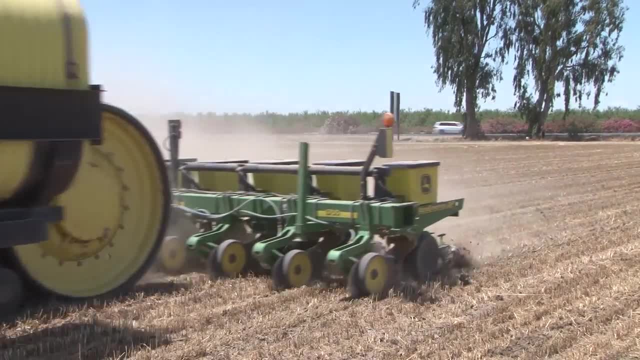 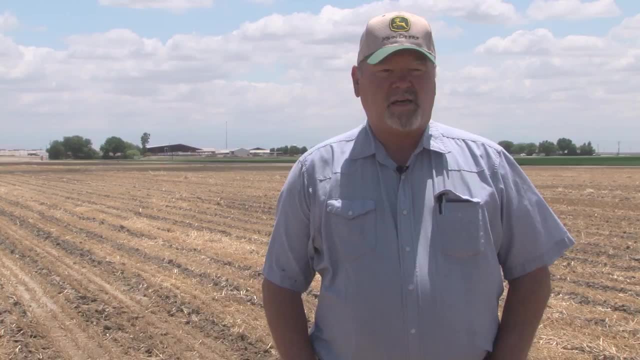 our equipment portfolio has actually shrank considerably from where it used to be, when we had to have multiple discs, lister bars, chisels, cultivators and a wide array of various other equipment. After the second year, we had an auction. 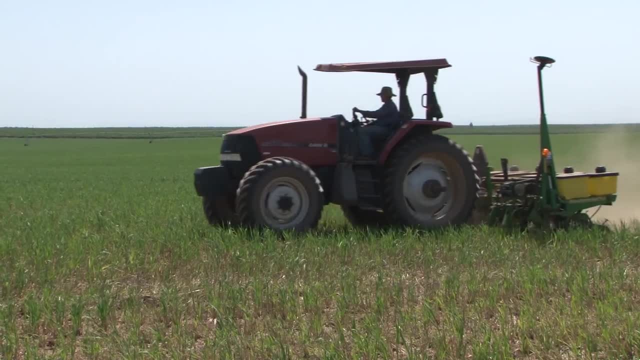 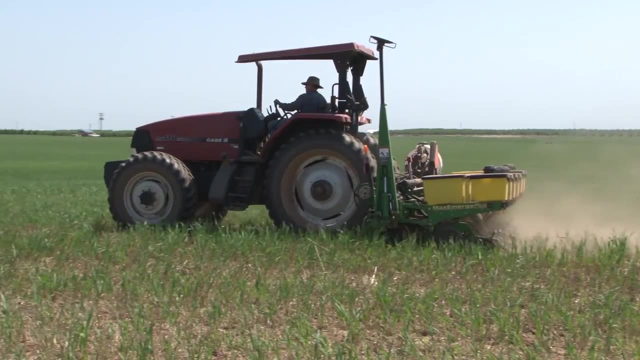 We sold all of our big equipment. Just sold it, Said that's it. We're not rolling any big equipment. We're not out there with any rippers. We're not out there with any discs. We're not out there with any chisels. 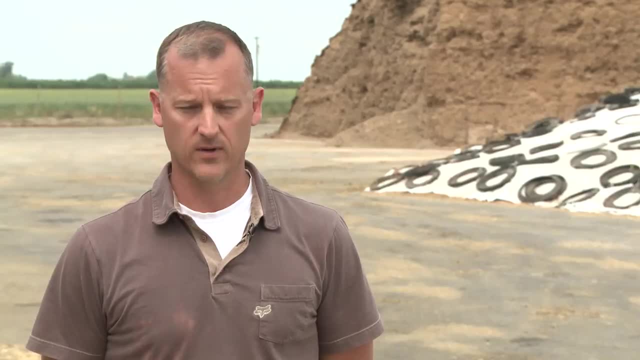 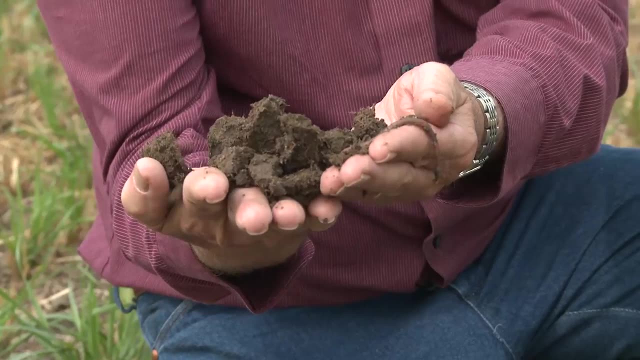 As we're finding out, when you put the time into it to understand it, there's definitely a potential there to be successful at no-till, When you can dig in this soil and you see earthworms just everywhere. To me, you see, this is beautiful soil because you smell it. It has that wonderful earthly 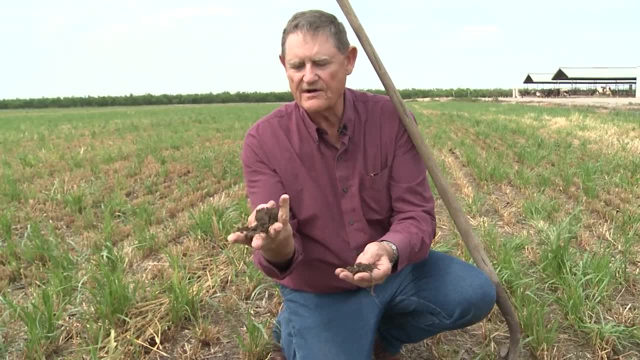 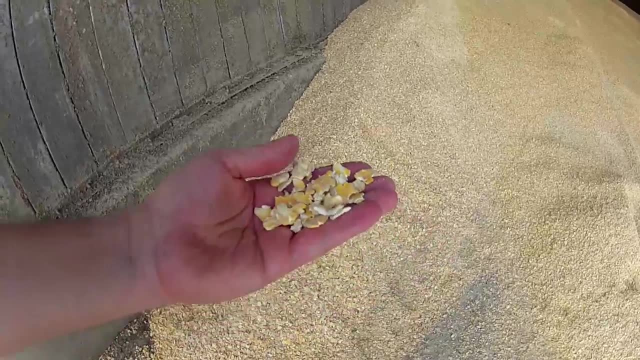 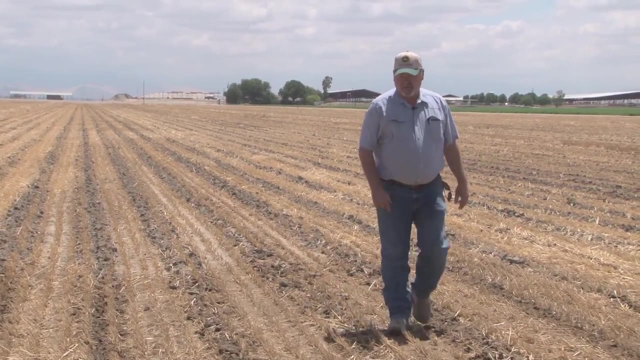 smell And you look at all the organic matter in there and that's all food for the next plant And we have seen increased quality of feed on the corn. Our quality in recent years has been better than it's ever been. As we look at this field here, it's already been strip-tilled. We have a nice small band. 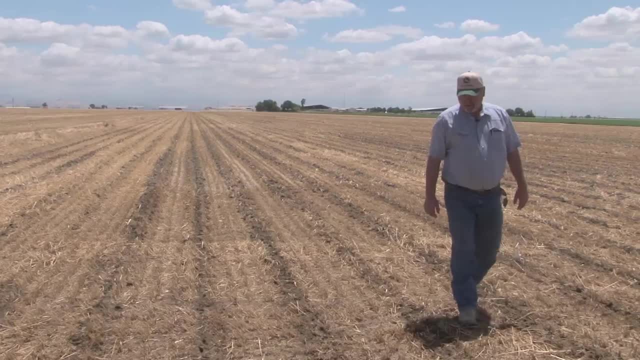 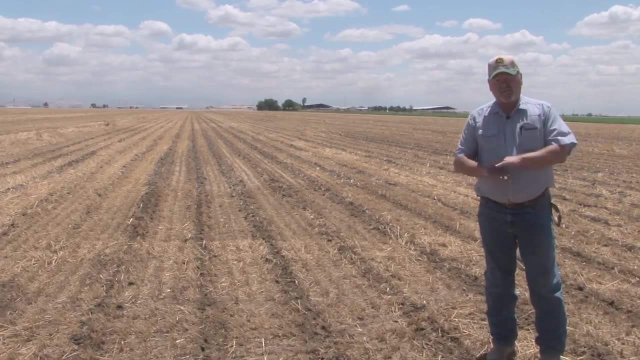 of perfectly tilled soil that's got excellent moisture. The strip-tiller did not raise too much soil. It's set just exactly right And when the planter comes back to the field right through and plants, it's going to be exactly level and it'll be perfect for germination. 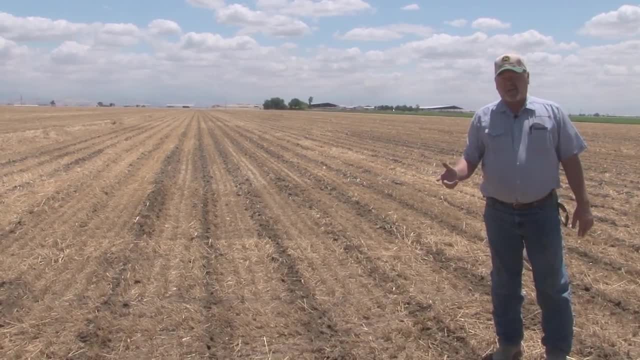 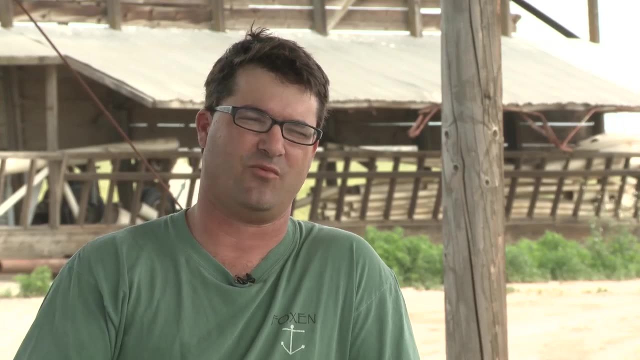 for irrigation and, most important, it'll be perfect for chopping later on, because all the ground is level. We're producing more crops now with less input, which is definitely a win-win. This is a typical John Deere planter, but it's been modified in a couple of ways. 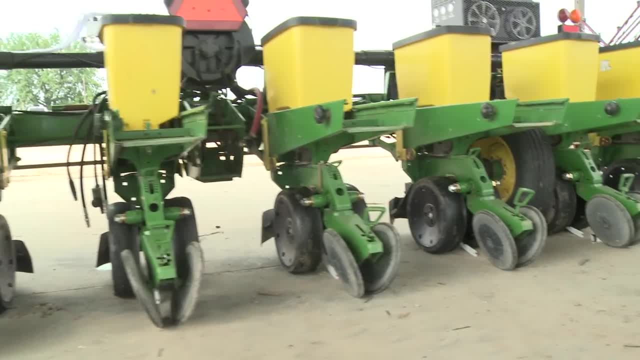 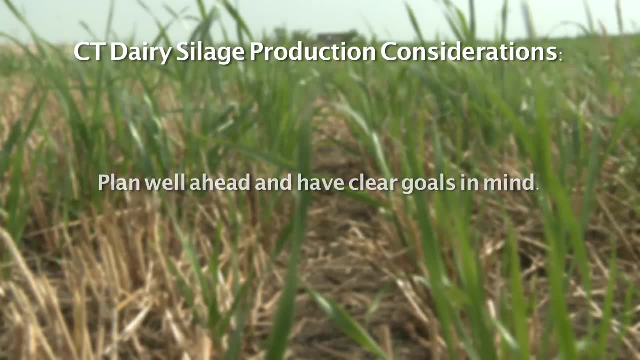 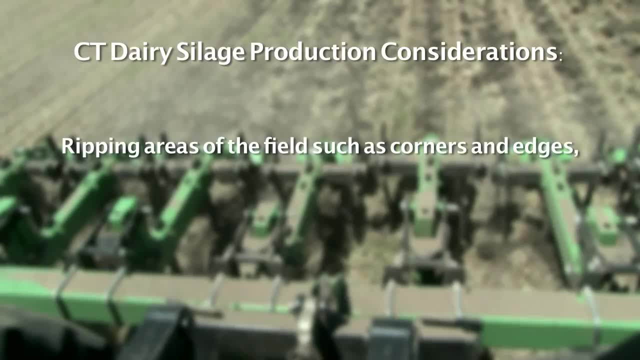 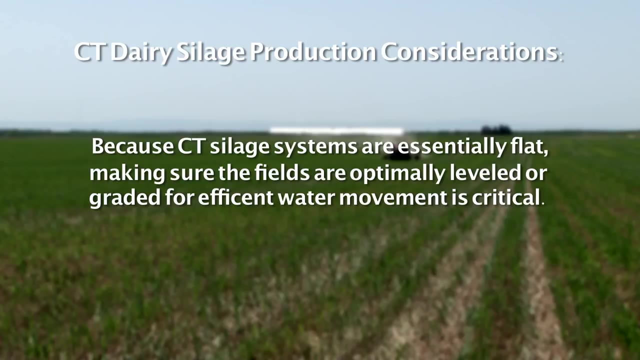 equipment. Ripping areas of the field such as corners and edges, where implement traffic patterns have been heavy and where sub-soil compaction may be an initial condition risk, may be useful. In addition, because CT salad systems are essentially flat, without raised beds, making sure the fields are optimally leveled or graded for a feedback. 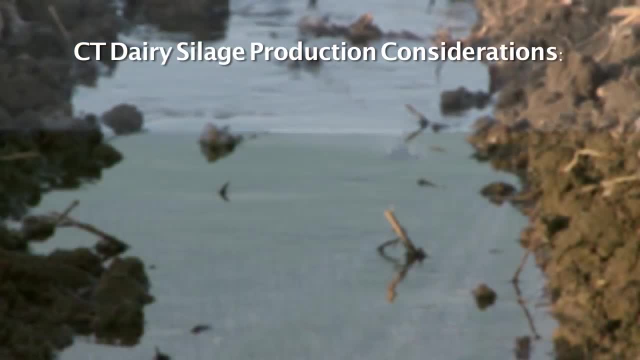 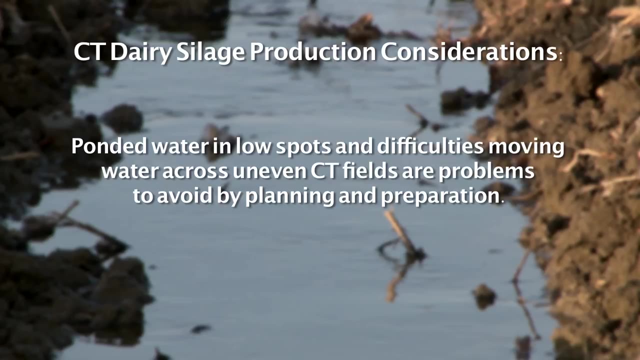 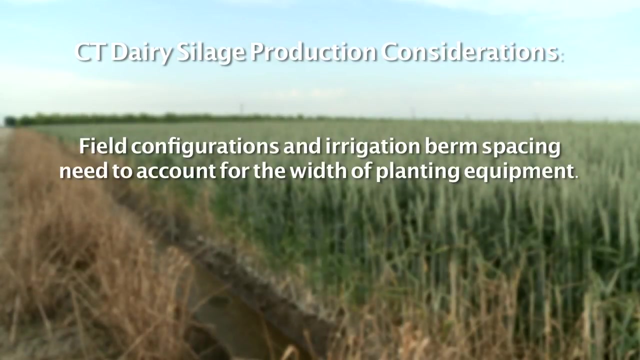 efficient water movement is critical. before getting started, Ponded water and low spots and difficulties moving water across uneven CT fields are problems to avoid by planning and preparation. Field configurations and irrigation berm spacing need to take into account the width of planting equipment that will be used. 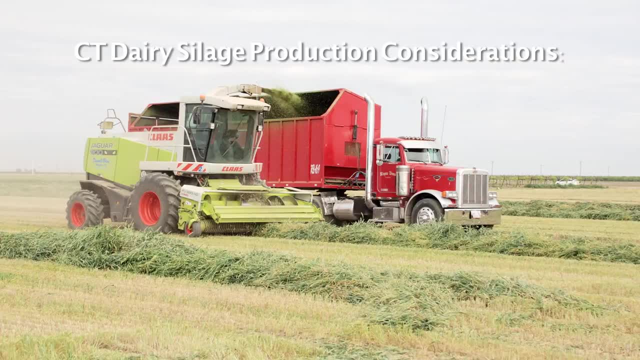 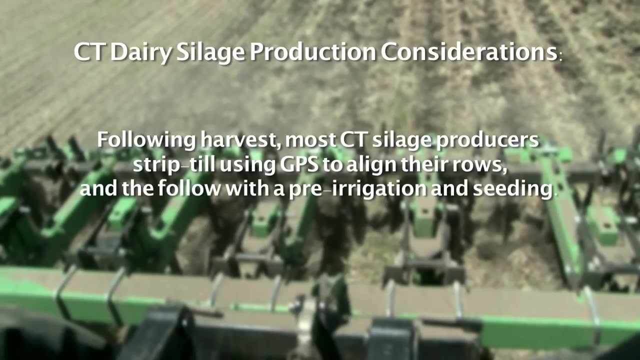 Following the chopping and harvest of winter small green silage. most CT silage producers then strip-till using GPS to align their rows and then follow with a pre-irrigation and seeding. Aligning the strip-tiller with the planter using GPS is critical. 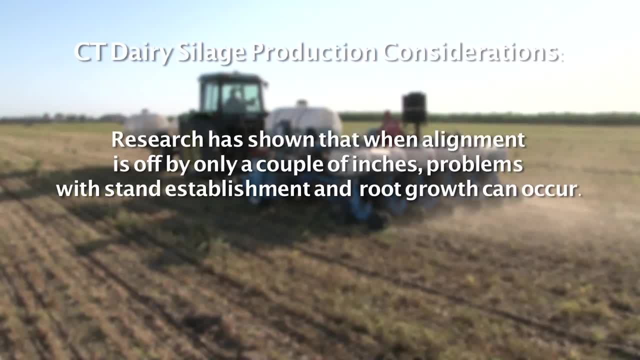 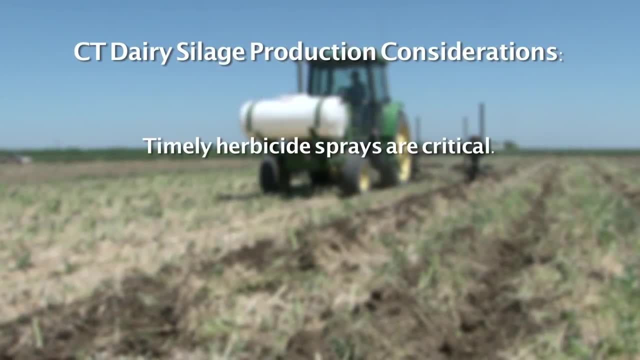 Research has shown that when alignment is off by only a couple of inches, problems with stand establishment and root growth can occur. Timely herbicide sprays are critical. CT silage farmers now recognize the need to spray early, often within a week of seeding. 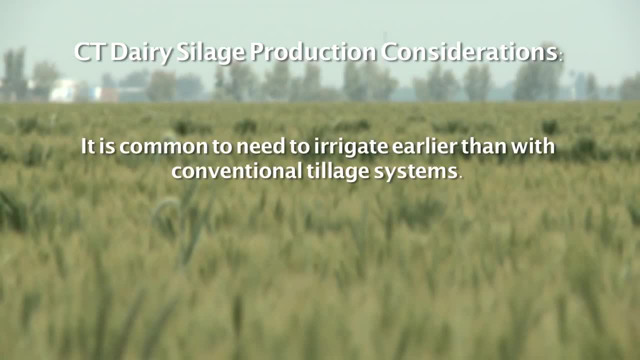 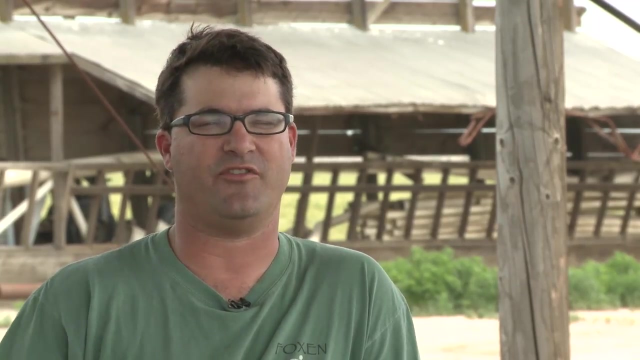 to keep weeds down. Lastly, it is common to need to irrigate earlier than with conventional tillage systems. Pay attention to crop needs, ET demand and soil water content to make sure irrigations are timely. I happen to know that every farmer that is involved in this process is more than willing. 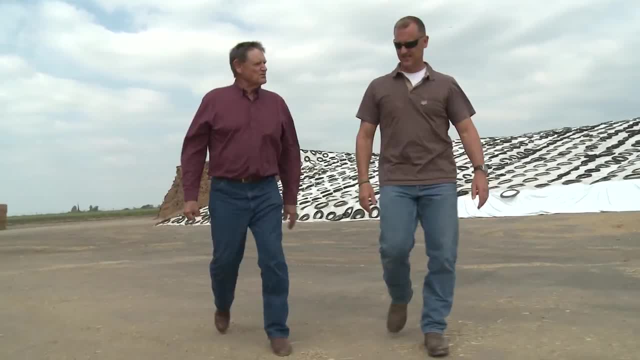 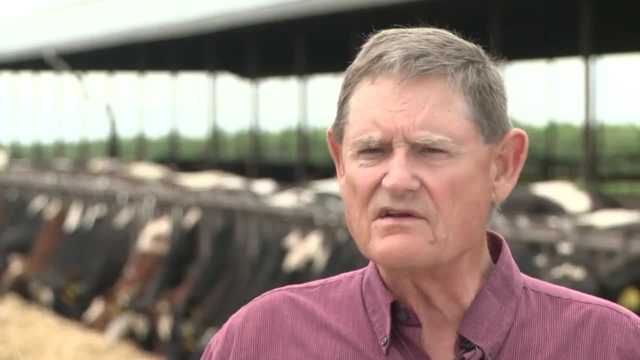 to share their experience. I've offered anybody anytime to come and talk about what they want to do and how they want to do it. I'll give them any input you know and be more than glad to You know when you compare. 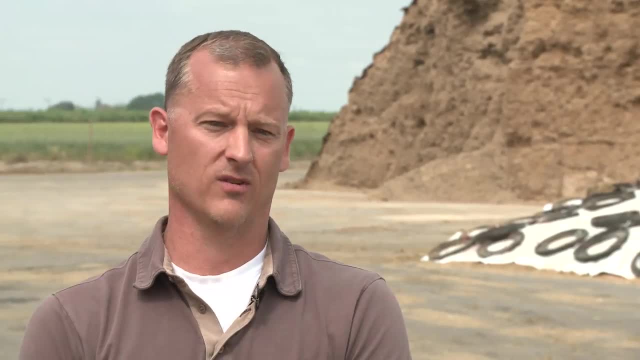 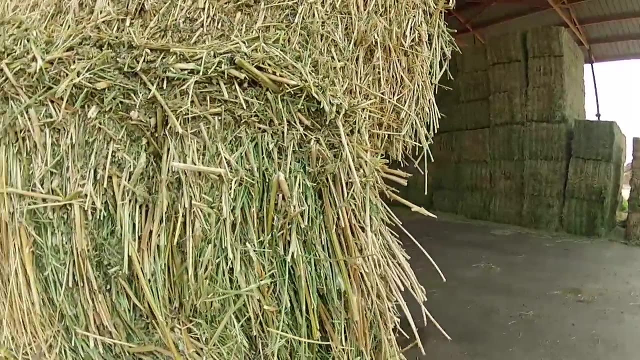 No-till or minimum-till to conventional farming program. you just can't compare the two when it comes to environment and cost savings. We've been at it about six years. I'm fascinated by it. I'm truly, I'm hooked. 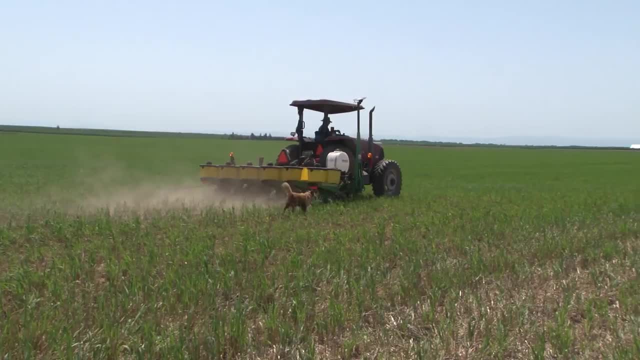 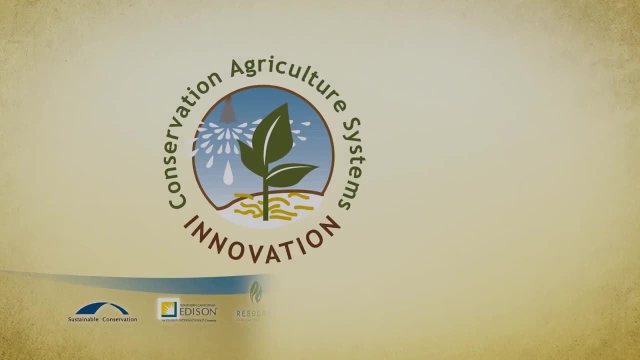 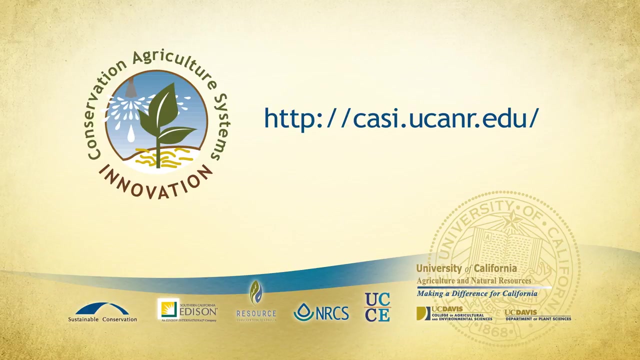 I'm hooked on no-till. It has all these benefits. They just become more and more visible every year. Additional information about these innovative conservation agriculture systems is in the description below. For more information, visit our website at wwwconservationagriculturesystemsinnovationcom. 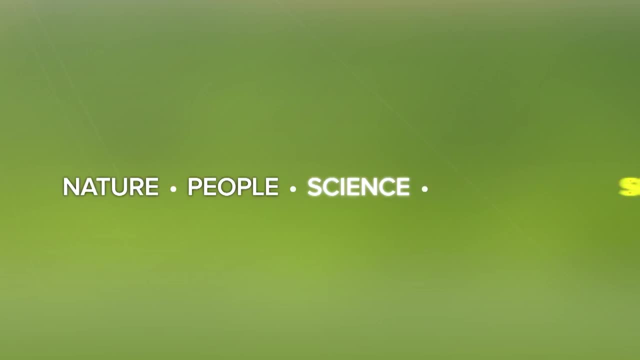 For more information, visit our website at wwwconservationagriculturesystemsinnovationcom.